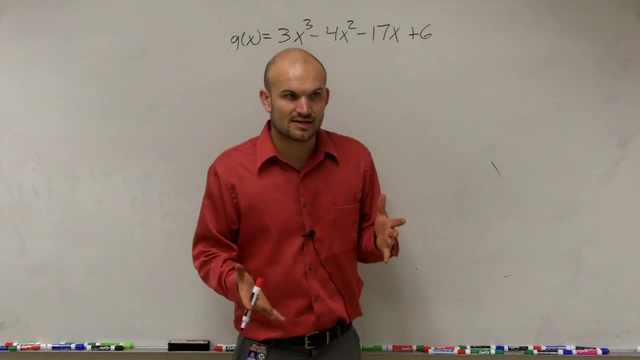 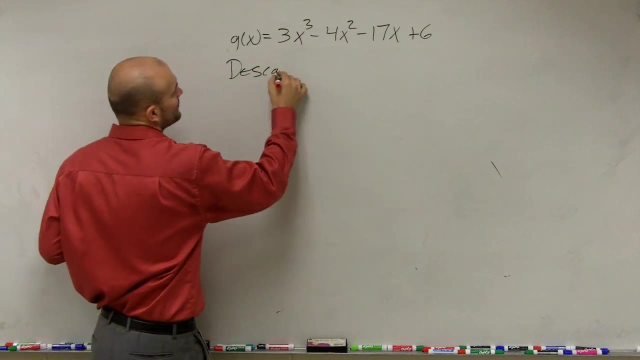 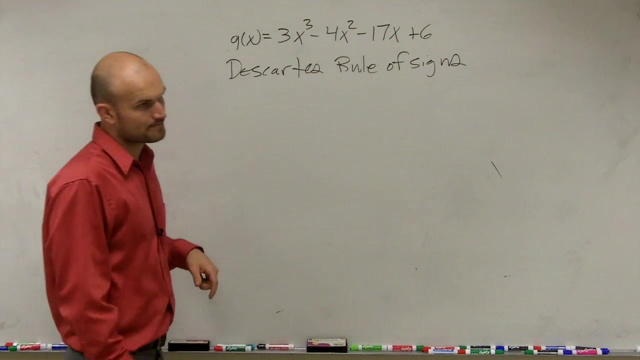 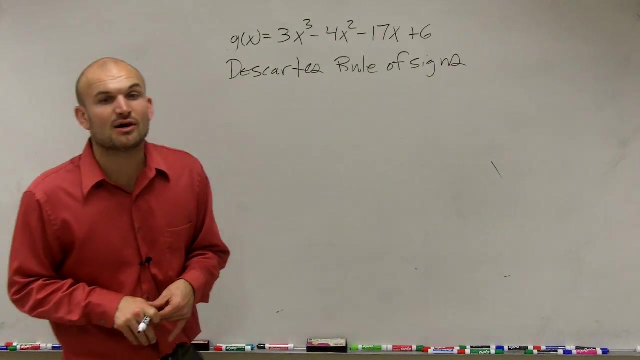 Well, there's another test we can use that's going to help us kind of identify a little bit more about talking about our zeros, And that next rule is Descartes' rule of sines. Okay so, Descartes' rule of sines. what this tells us is the number Amber of positive and the number of negative real zeros. 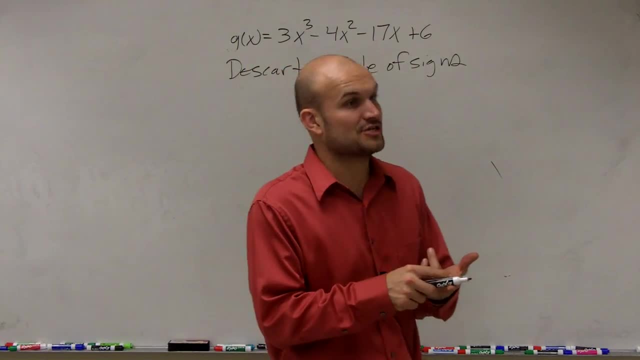 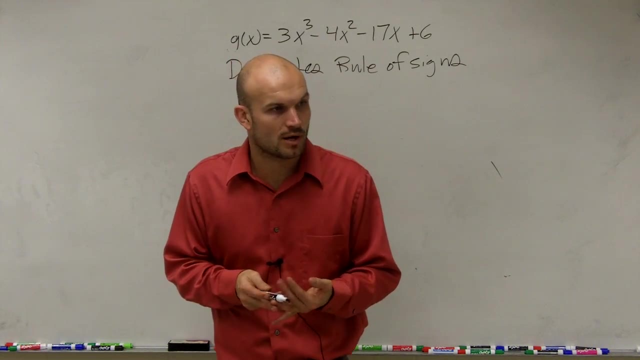 So now again, we're just going to be talking about real. but real can be imaginary, I'm sorry. Real can be irrational, and it can also be irrational and rational as well, All right, So how does Descartes' rule of sines work? 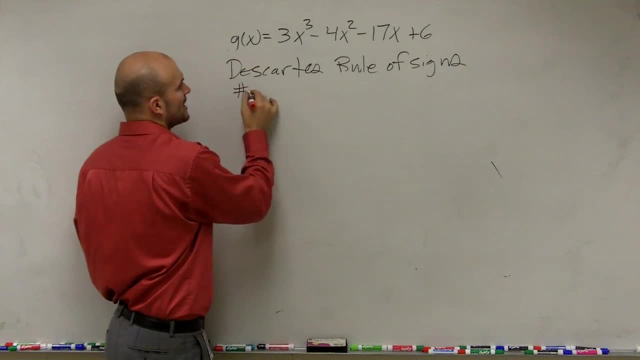 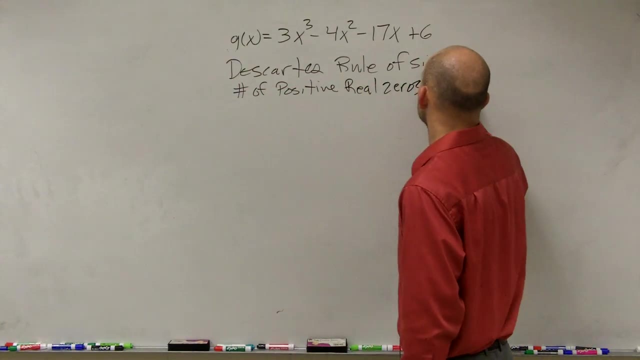 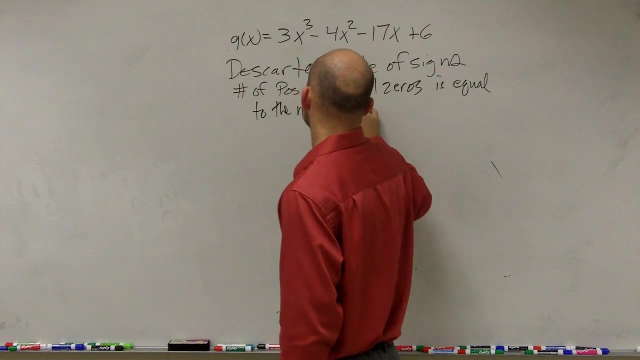 Descartes' rule of sines is going to say: let's first find out what the number of zeros is. Let's first find out what the number of zeros is, Let's first work on the positive, So we're going to have the number of positive, real zeros is equal to the number of sine changes. 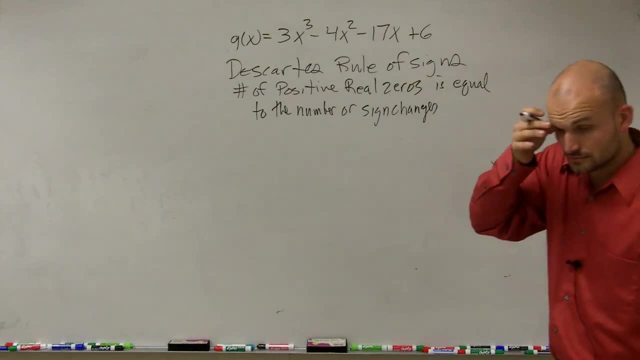 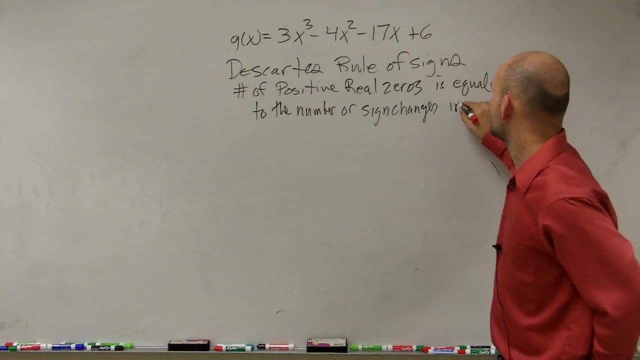 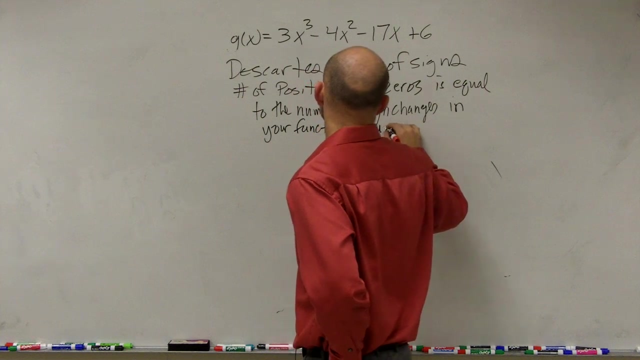 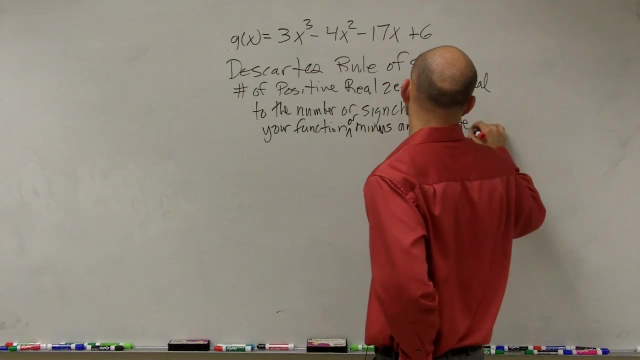 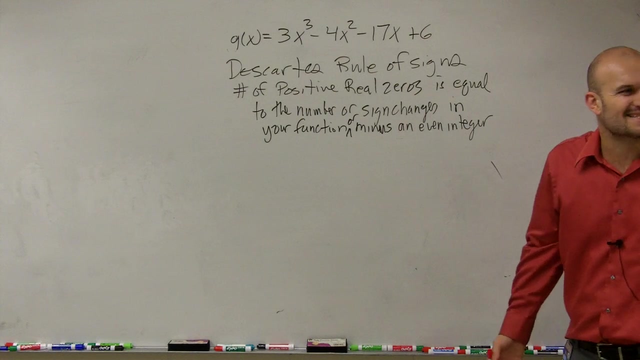 in a polynomial or in your function, minus or minus, an even integer, And I'll explain that in a second. All right, So let's go and take a look at this. So let's look at, in this first problem, how many sine changes do we have? 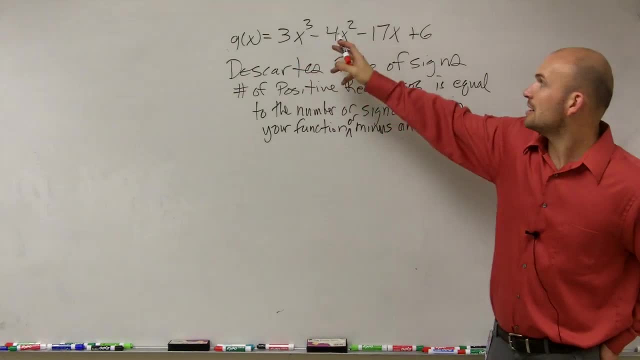 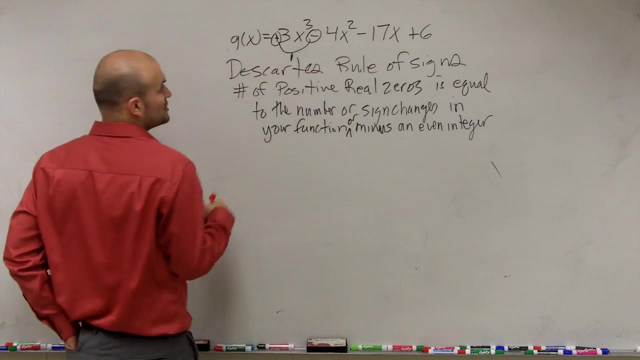 Well, our first term is what? Positive, And then the next one is negative, right, So we have one sine change and then we go from negative to negative. That's not a sine change. And then we go to negative to positive. 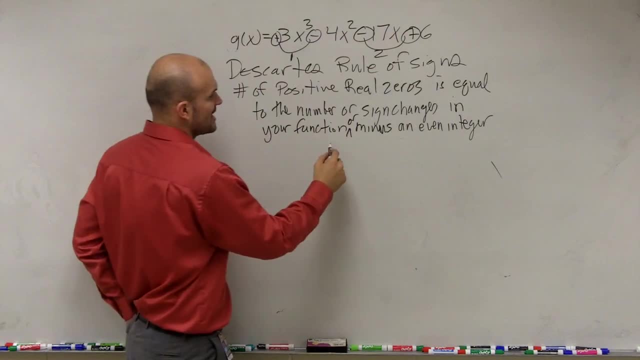 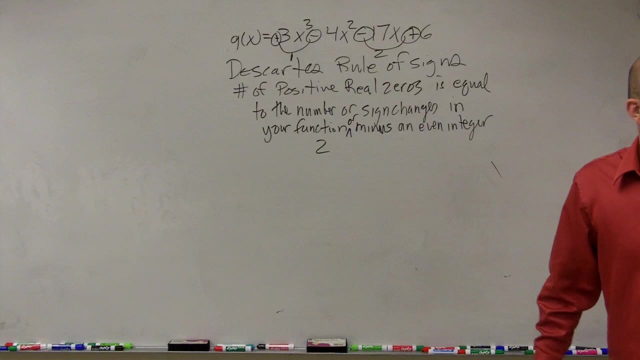 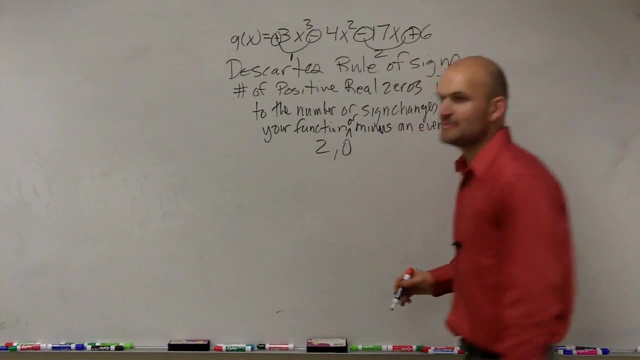 So that's two sine changes, right. So we could say there's two positive zeros or minus an even number, which the sine changes are. The smallest even number is two, right. So two minus two is zero. So that means there's either two positive real zeros or there's none. 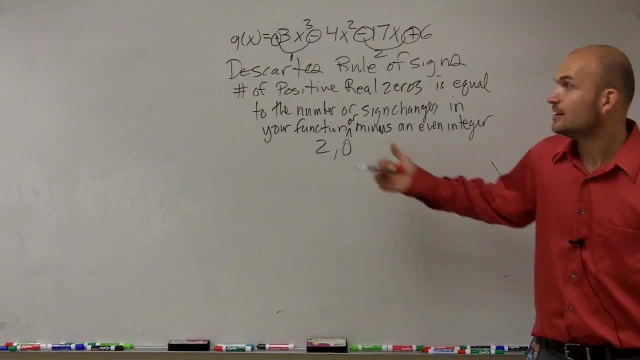 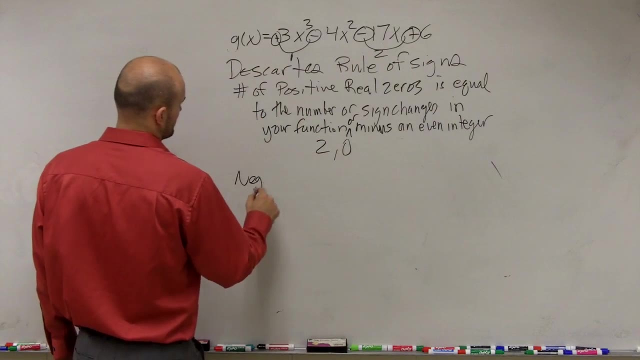 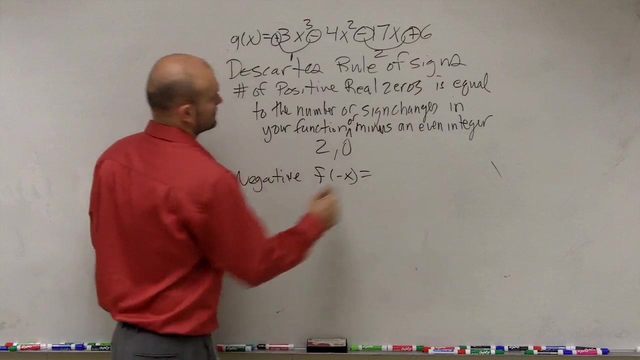 We don't know which one yet, but we know that by this test we're not going to have one real zero. All right, Then the number of negative is the exact same thing, but for f of negative x. So let's do f of negative x.